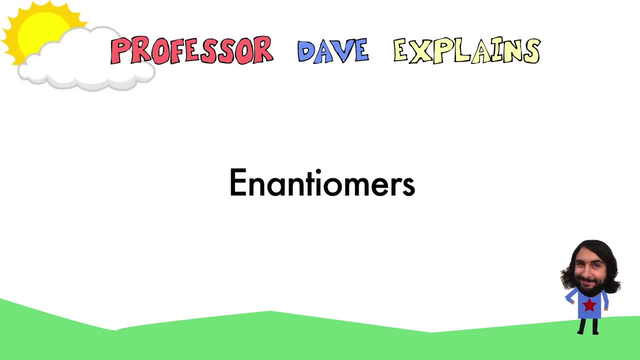 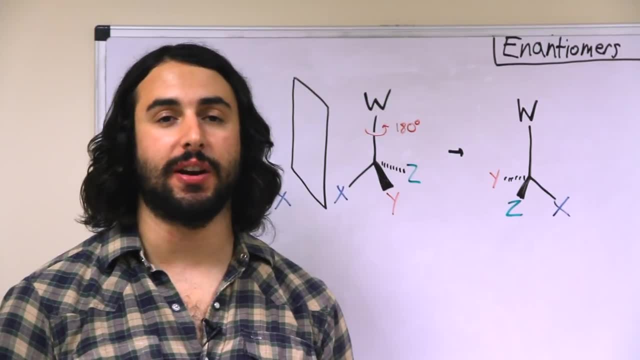 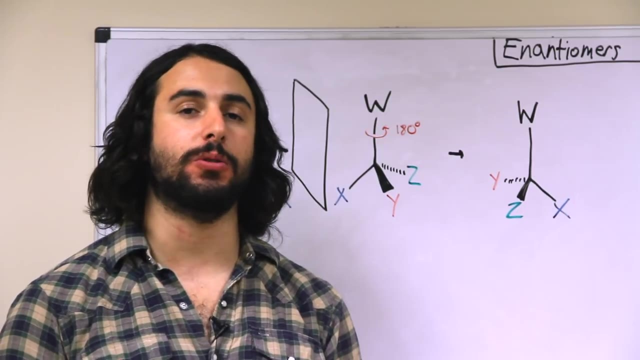 And let's talk a little bit about why. So the first kind of stereoisomeric relationship I want to talk about involves molecules that are called enantiomers of one another. Enantiomers are molecules that are non-superposable mirror images of each other. 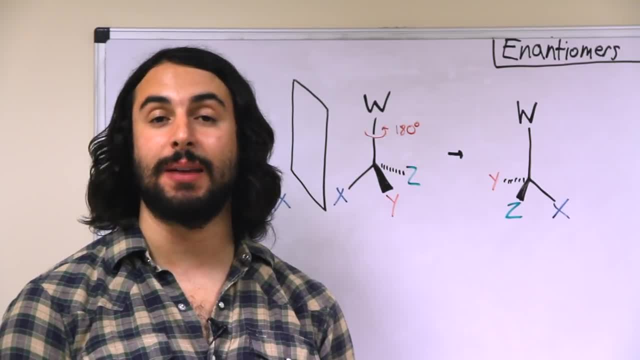 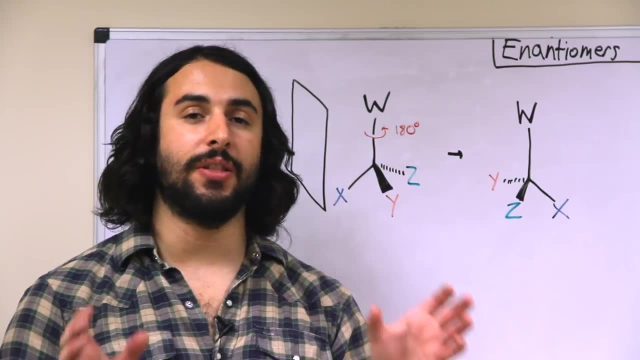 In other words, they are stereoisomers, so they have the same connectivity. But if you take the mirror image of one of the compounds, you get the other and they're not the same because they do not overlap precisely the same way in three-dimensional space. 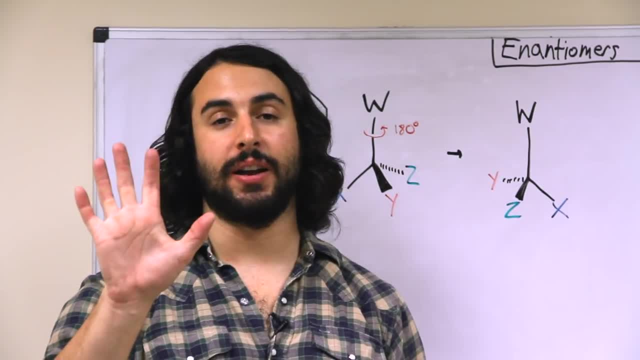 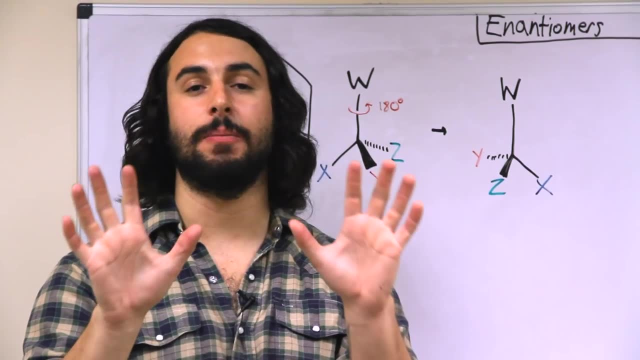 So take for an analogy our hands. So here's one of my hands, and the mirror image of this hand is my other hand, right? So these have an enantiomeric relationship in the sense that they are mirror images of one another. 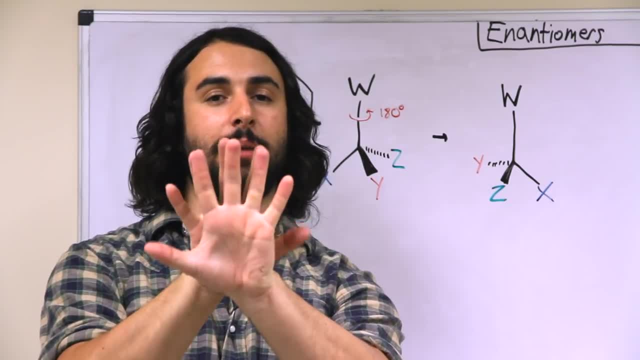 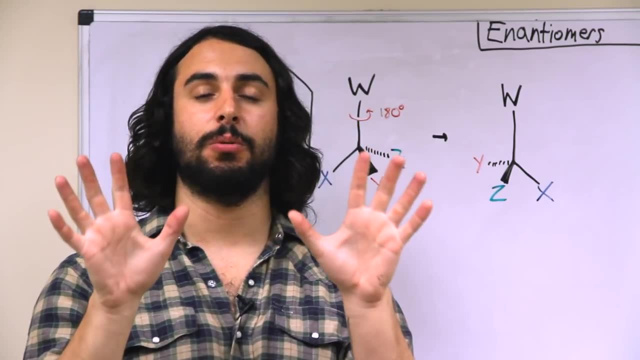 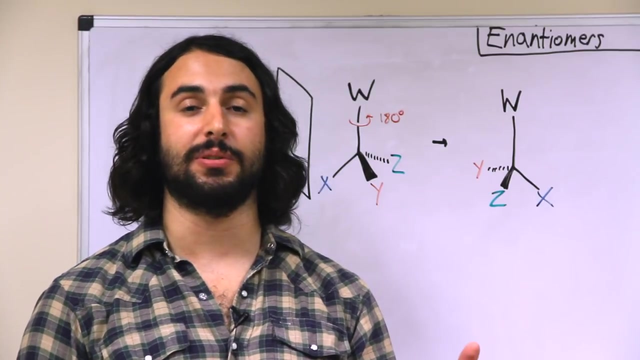 but they do not precisely overlap. I'm not going to be able to get every finger to overlap its corresponding finger properly. So they have an enantiomeric relationship because they are non-superposable mirror images of one another, And we can come up with all kinds of macroscopic examples of this. 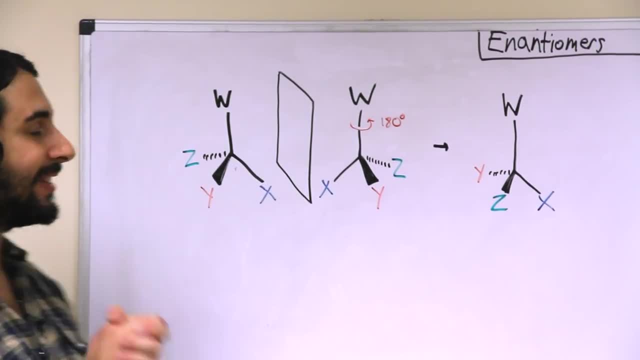 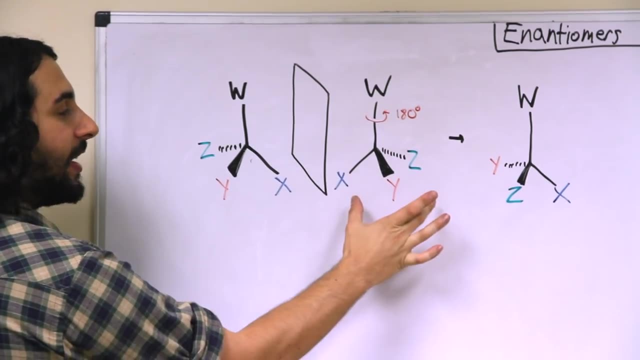 But molecules are doing the same thing. So let's take something like this molecule and let's reflect it across a mirror plane here, And we can all agree that this is the mirror image of that, right? So we have X. whatever these atoms are, it doesn't matter. 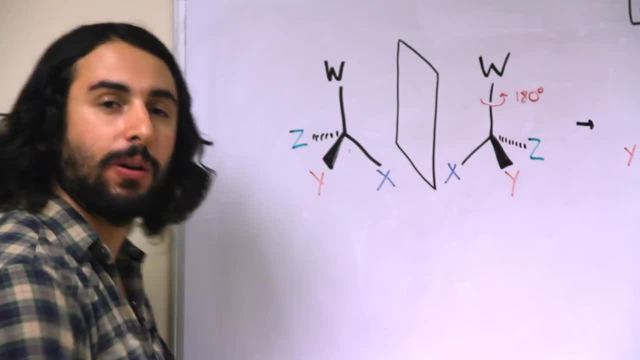 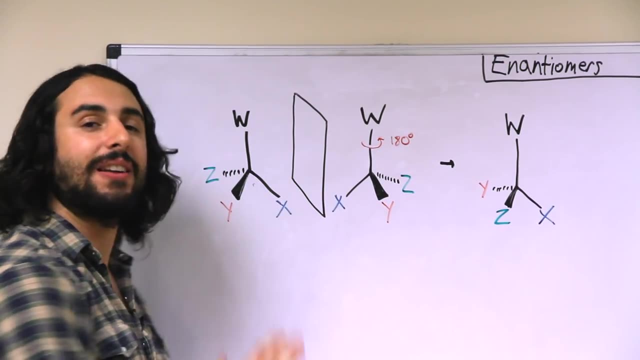 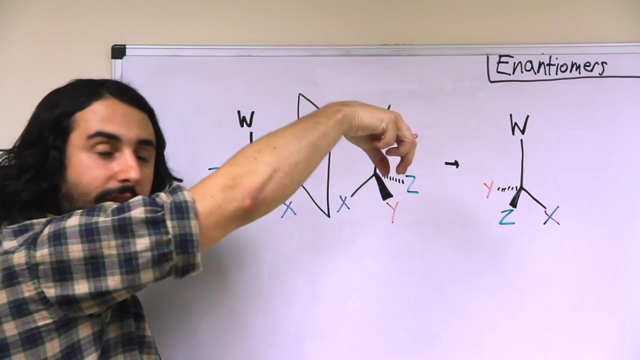 X and then the Y and then the Z. these are mirror images of one another. But now if we rotate the resulting mirror image to try to place it on top of the original. so in order to do that, if we want the X to line up, we're just going to twist this like a top 180 degrees. 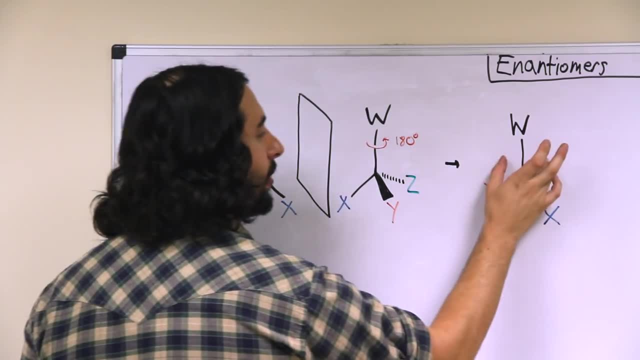 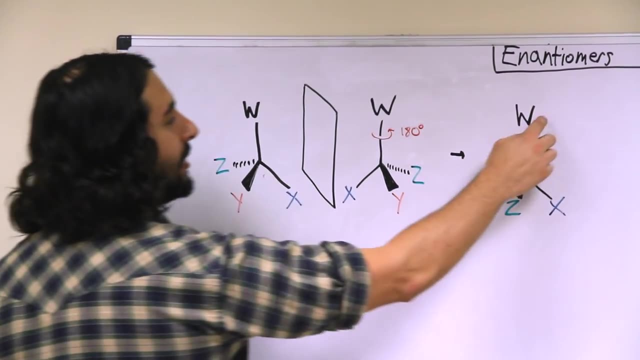 and we would get this. But the problem is, if we try to take this and put it on top of that, not all of the atoms are going to overlap properly. So the W, the central atom, and the X, those would overlap just fine. 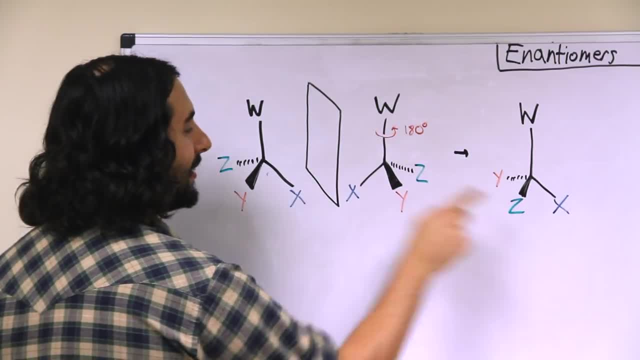 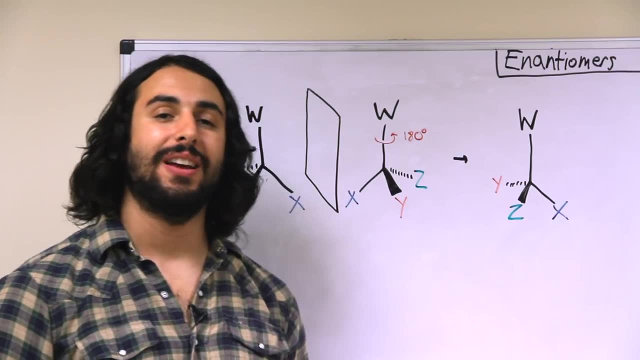 but you'd find that the Y would just overlap, The Y would be on top of the Z and the Z would be on top of the Y. Therefore, these, this molecule and its mirror image, which are two distinctly different molecules, are enantiomers of one another. 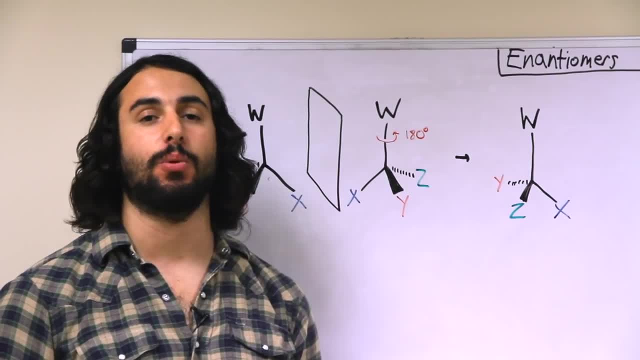 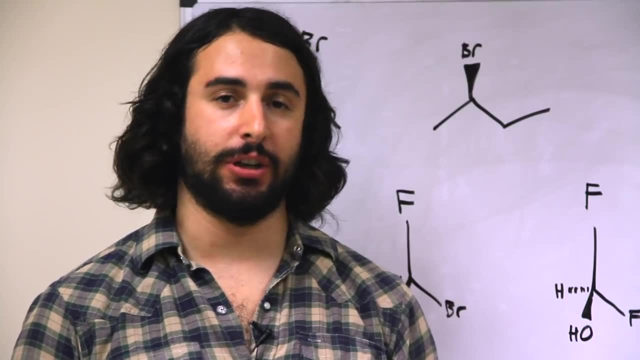 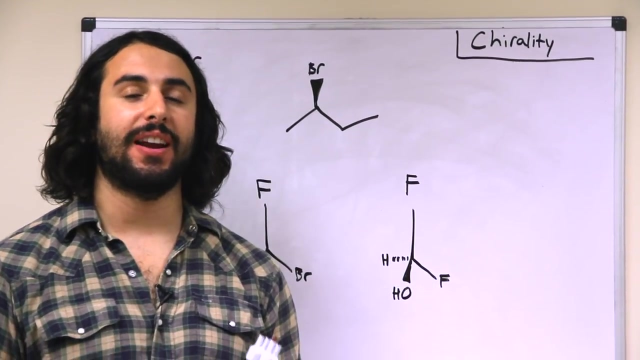 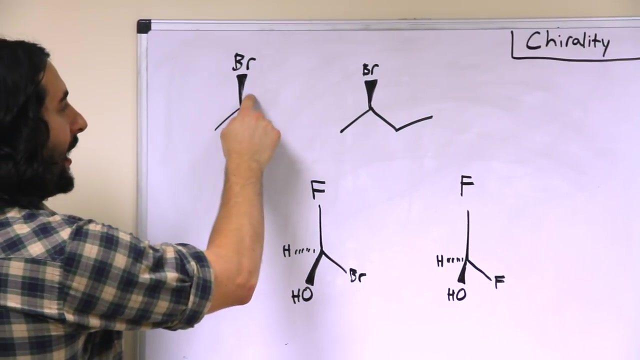 because they are non-superposable, mirror images of one another. So molecules that have an enantiomer display a quality called chirality. This is something that we would typically assign to a carbon that has four different substituents projecting from it. So, for example, on the top, this carbon atom has a bromine atom. 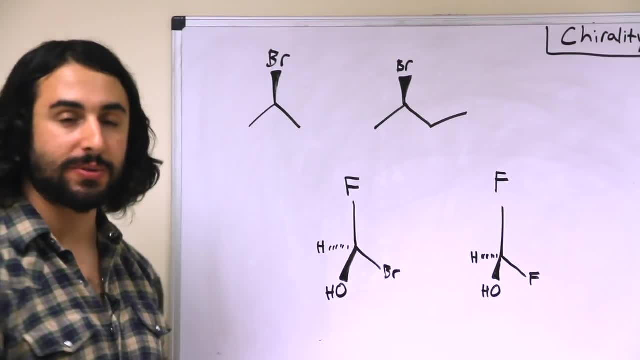 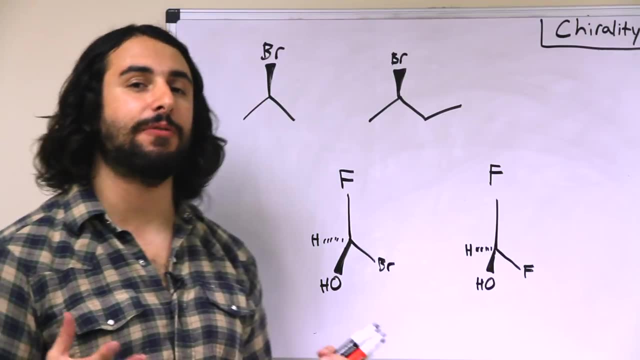 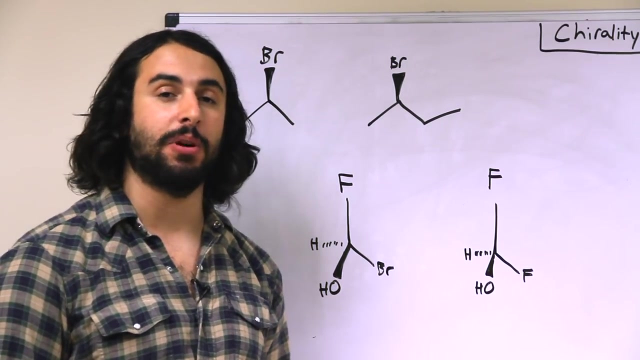 the implied hydrogen and two identical methyl groups. So we would not regard this as chiral because it has two identical methyl groups, so it does not have four distinctly different substituents. Now this would mean that this does not have an enantiomer. 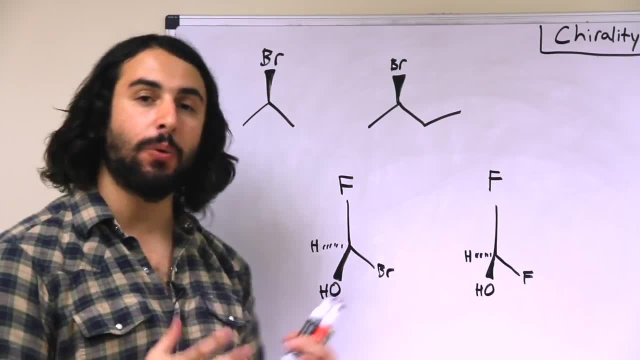 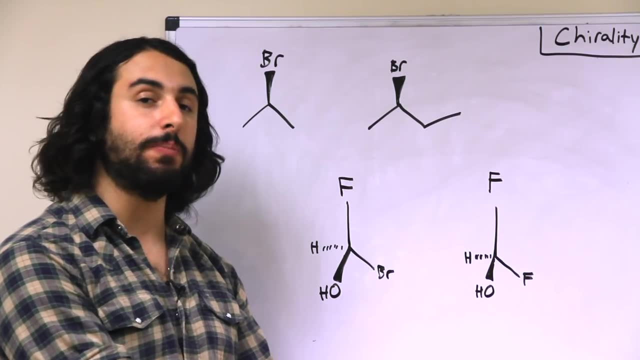 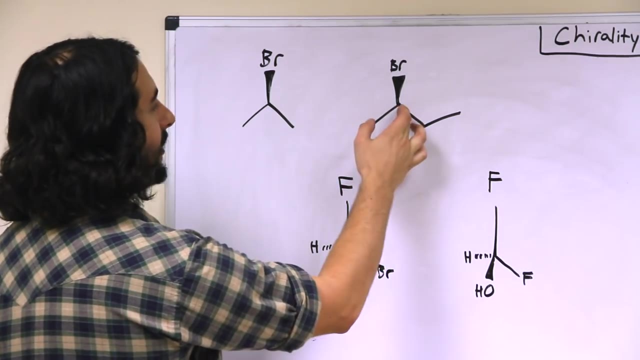 because if you made the mirror image of this molecule, it would be precisely the same molecule. it would be superposable, so it would not have an enantiomer. its mirror image would be identical and it is therefore not chiral. However, this molecule is chiral because this carbon has a bromine atom. 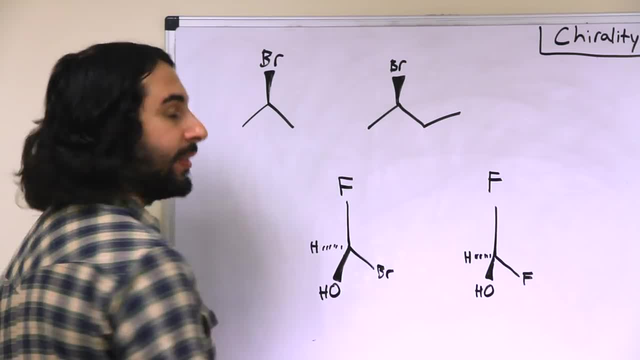 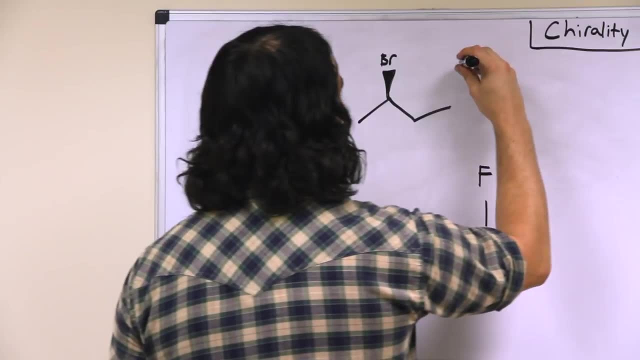 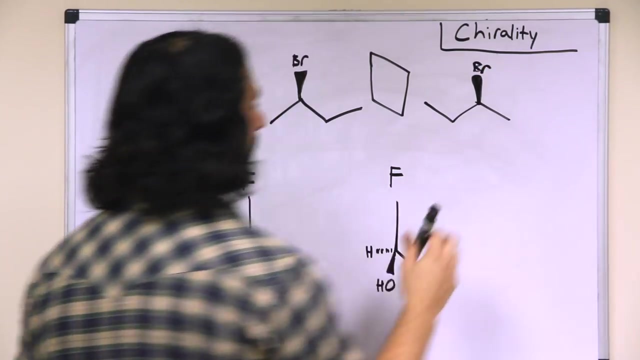 the implied hydrogen. this one carbon chain and then a two carbon chain. So that is four distinctly different groups, and if we went and took the mirror image, we would see that it is that. and now, if we try to flip that around, 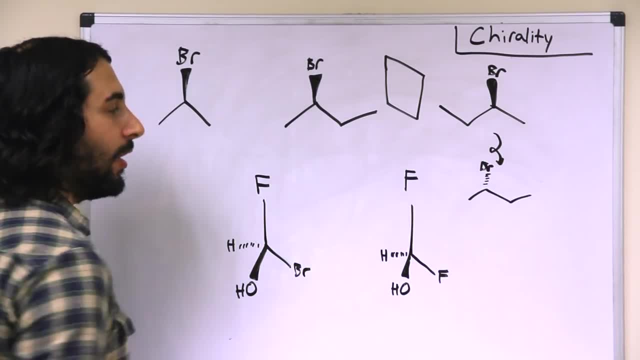 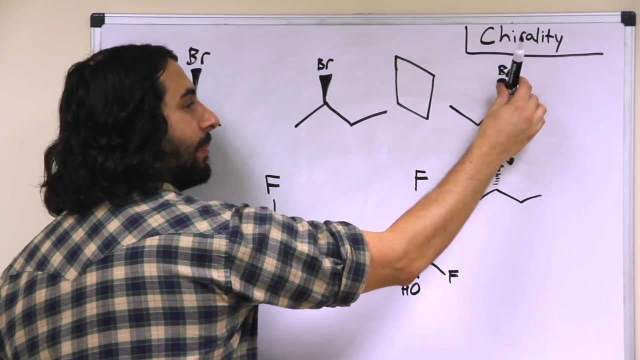 we would get the same structure, but now the bromine would be on the dash bond, because if the bromine atom is on the wedge bond out of the board like this, if we flip the whole thing 180 degrees now, the bromine is going to be going into the board. 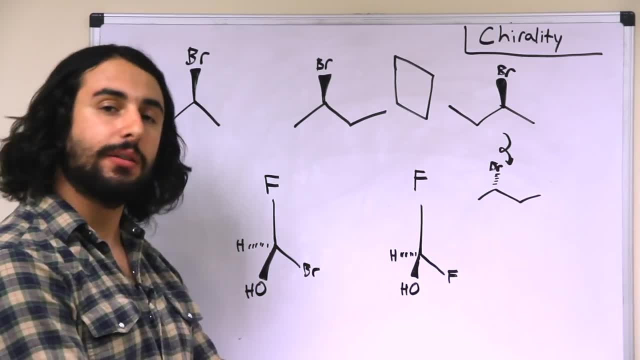 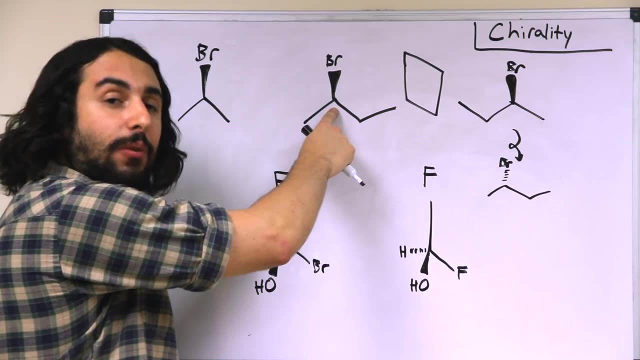 so if we try to place this on top of that molecule, it is not going to line up properly. so therefore, this molecule is chiral, it has a chiral center, or a center of chirality, or a stereogenic center- all terms that mean the same thing. 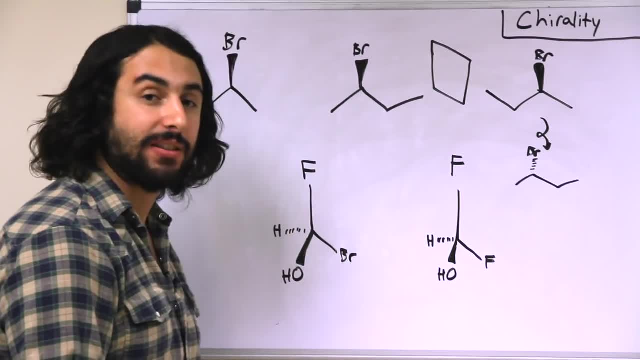 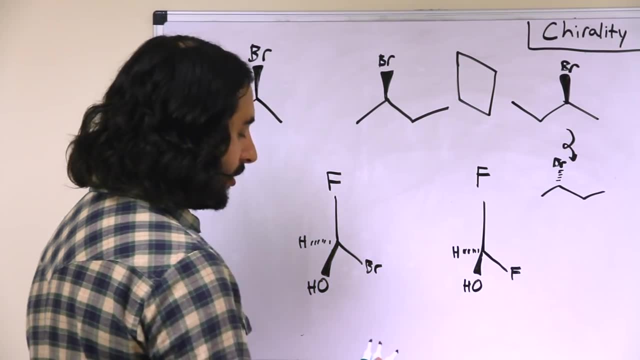 and therefore it does have an enantiomer. Likewise, over here this is a carbon with four different groups. this is a similar molecule, but two of the groups are the same. we have two fluorine atoms. So if you at home want to go ahead and check.